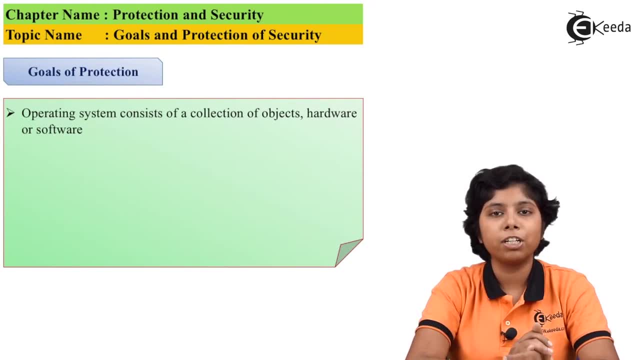 becomes an extremely crucial one. while we are configuring the network management of that operating systems, transferring data to other operating system or other machines. Now, when this type of this operating system transfer done, then a healthy subsystem of that operating system can get infected by a malicious program, into a virus infected. 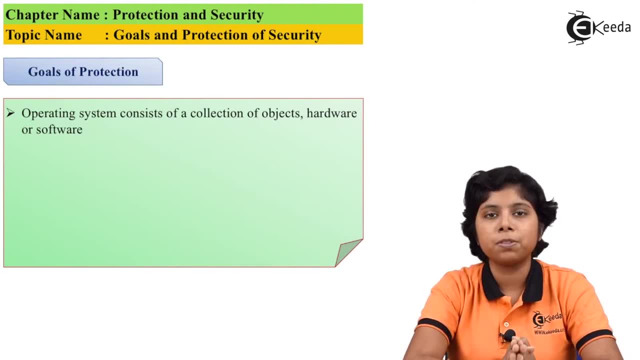 malicious system. So we need to avoid this type of systems. that is the reason for giving protection to the data and information inside that system. So, while we are giving protection to it, so we must mention that the user first need to be authenticated. that is the first need of protection. If the user is an unauthorized user, then the 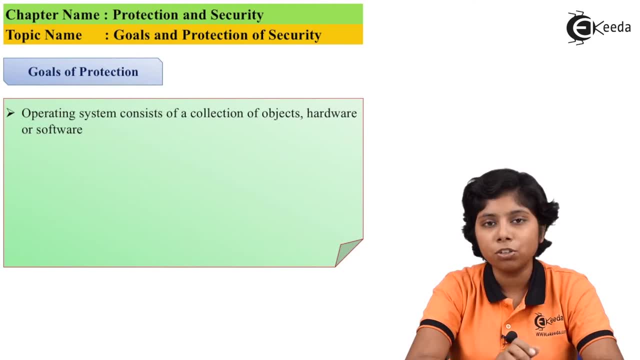 message that is coming for it or any access right that is given to use that resources of the system is no meaningful. So first need for the protection is the user authentication. The second need is that the files and the data that is stored should be done. 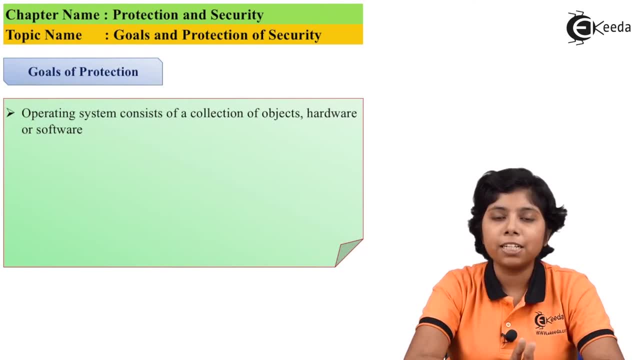 in an consistent and conveniently Say, for an example, that all the files that are stored within a computer can be accessed by any of the user of that particular operating system, so that the files are not secured and shared by any user, so they can be modified by any of the user. so the owner files which are 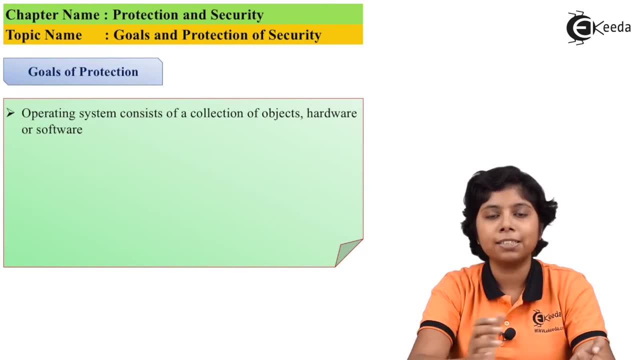 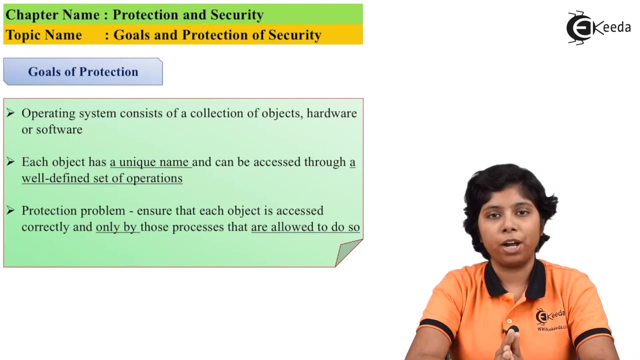 for only the configuration purposes and now can be accessed inside this users, which has only the read and write operations. so this should be done in the need of the protection. now the third need of the protection is to protect the users of their own files and programs. say, for an example, a user 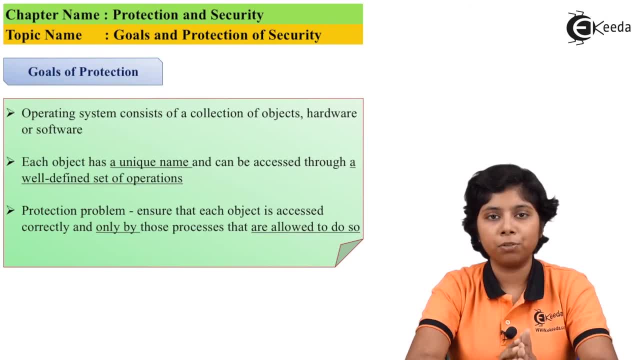 is having its own files and protection codes on that particular files. so if the protection codes are not there, then any user can access to the files without granting an elevation by the user which is owning the file. so this need not to be done, and that is the third reason for protection. 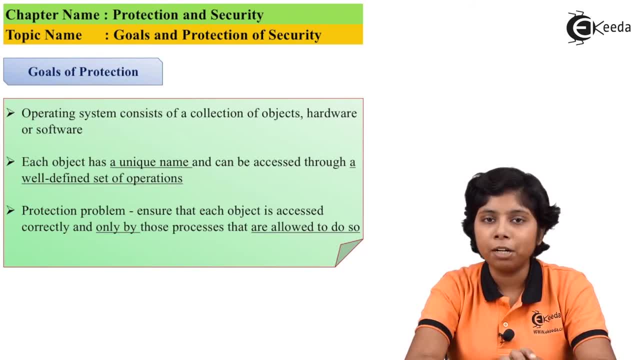 so the providing protection, information and environment to a file and instead of to the environments types, so that the user can protect themselves from other users and the user can access the files without the user's permission. so this is the third reason for protection, as well as an important actors of the operating system. so the protection policy should be there. 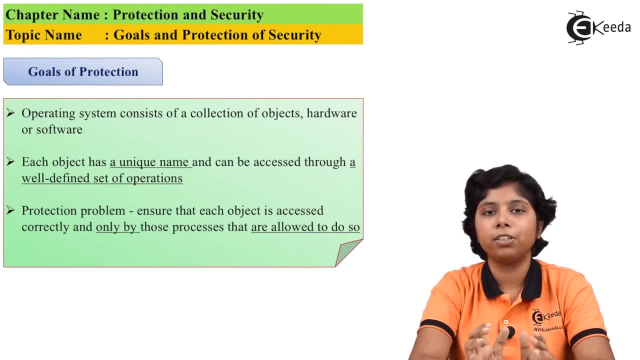 to determine that what is the protection that need to be done on that user's file? so if it is a common file, then it can be accessed by any of the user and if it is a private file to the user, then it need to be protected with the executable mode so that the policies can be changed from time to time. 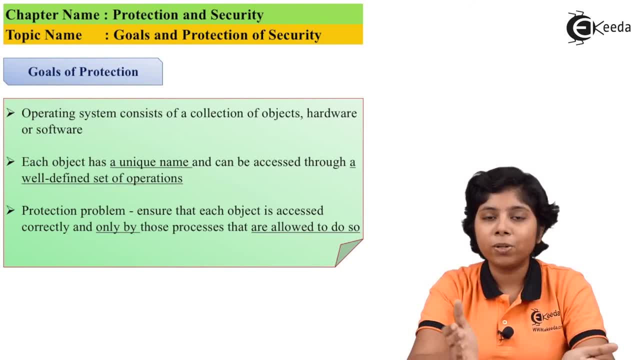 and can vary on from the application to application. so it is not the sole responsibility of the operating system designer to take care of the protection. the protection is needed to be done on the application programmer side too, as the application can vary between the protection needs. so the application programmer or the system designer must specify that what are the protection? 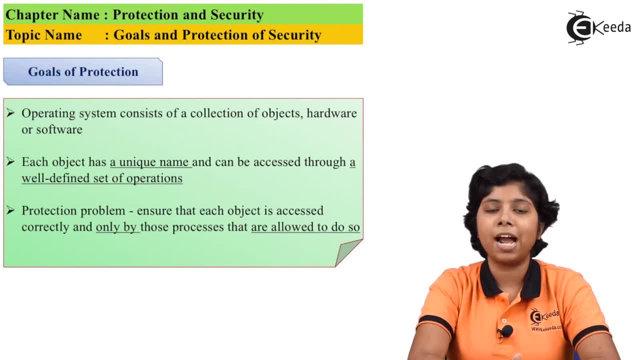 that need to be taken care of while performing the application and that particular version of that application. so in this way and the protection can be taken and it is very much important for these factors to be taken care of. so if all these factors are taken care, then we can say that 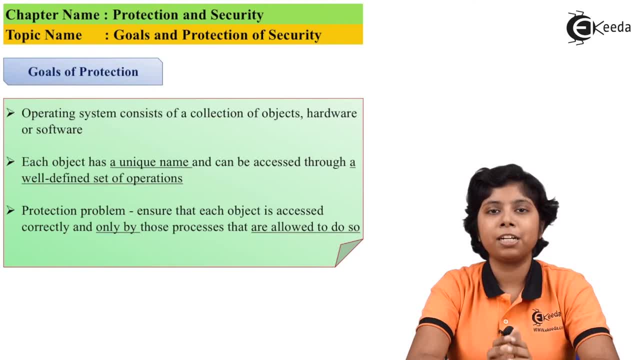 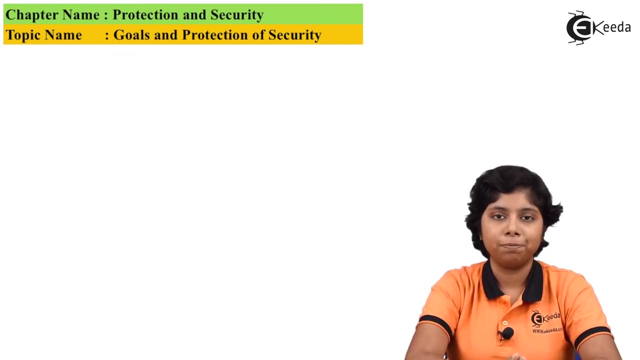 our system is secured and protected by mechanisms of protection. so the first one is user authentication. news is the user files and directories and healthy subsystem maintenance and also the application programmer interference in that particular protection policy. next we will move to our next part, that is, the principle of protection. 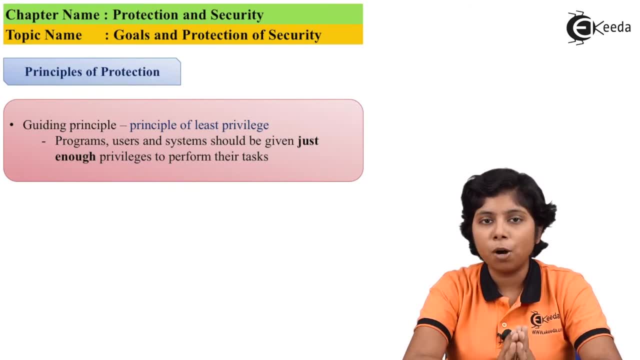 the main principle that is adopted by most of the operating system to protect their environment at from a computer's end is to maintain the least privilege policy. while the computer operating system maintain the least privilege policy, it is telling the users that only the privileges that is need to access those files will be given to the user and other than the user cannot access any of. 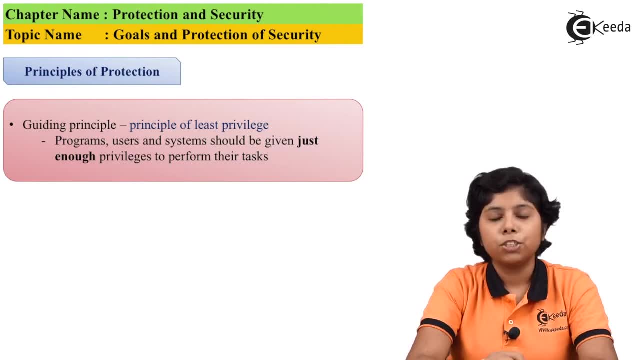 the files on that particular file system or operating system. we must first distinguish between the policy and the mechanism. the policy is what to be done and the mechanism is how it is to be done. so the first distinguishable between this policy and mechanism gives us the flexibility to protect an environment. so even for an vote scenario, every policy will 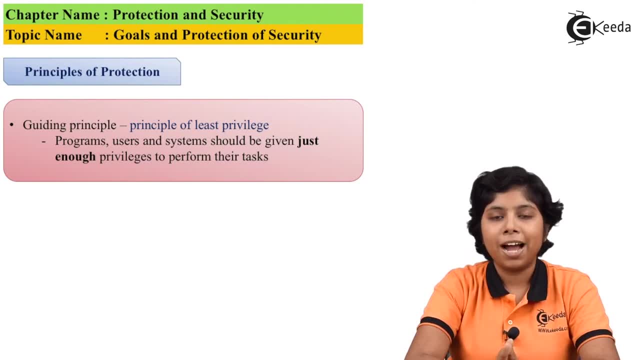 require an underlying mechanism to change in every way other than that a policy is fixed and there are many mechanisms to imply those policy according to the policy that is being implemented, in the same way that the policy requires the implementation of a policy be followed which allows the 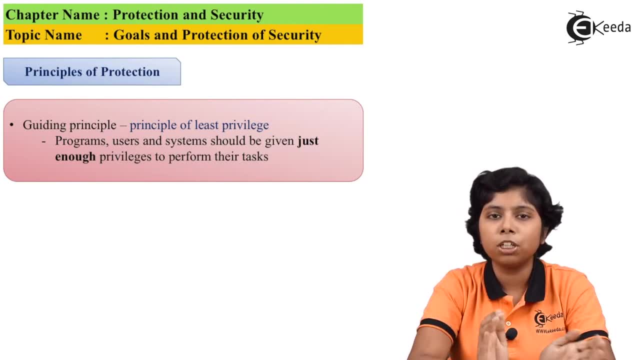 flex trên mins and the policy environment that is being constructed to protect all possible sources of the security. key. security guad is secretly security. past key equals security is precedence, because one key is associated with many of the areas. so in like this way the access privileges walk in operating system there. if one access is given to all the user, then the mislead. 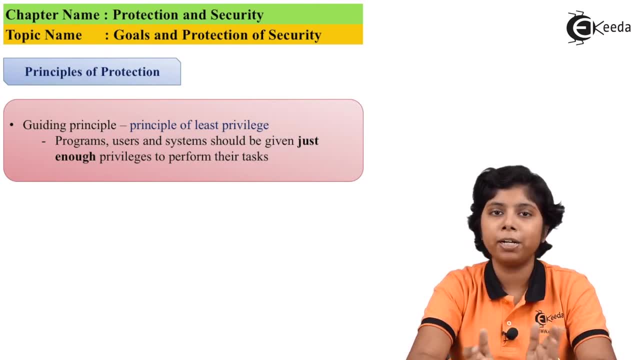 of this and misinterpretation of these access privileges will be done by the user. so we need to follow the principle of least privileges that is accommodated by this user operating system. so they are provided a role-based access control or rbac protocol. this role-based access control. 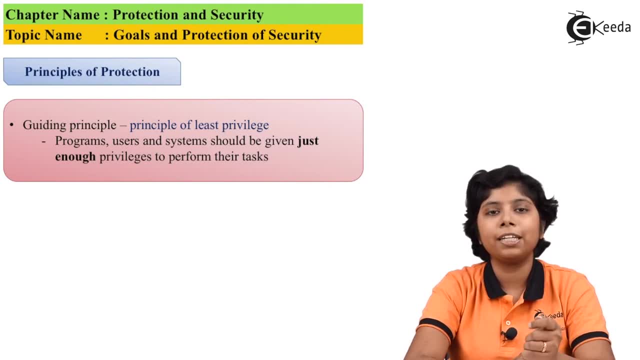 enables that a user should control only in their owner or user or universe way to access control on that particular file. say, if it is the owner of the user, then it can read, write and execute a file. if it is only from the other group members, then it can write and write the files. 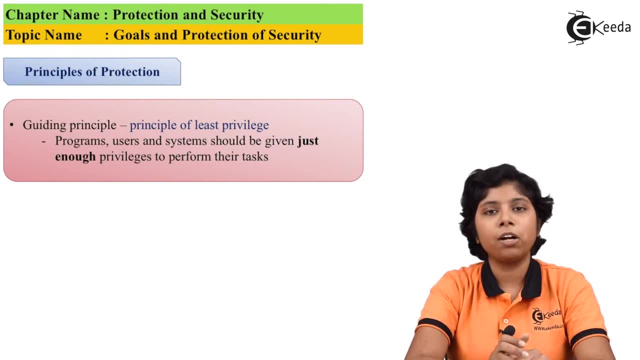 and if it is from the users or the universe, then it can only read the file. so according to this role-based access control, we can prescribe the acl to maintain a list that which user has which access rights or privileges to the user. now this list of privilege action principle can be intruded by any attacker which 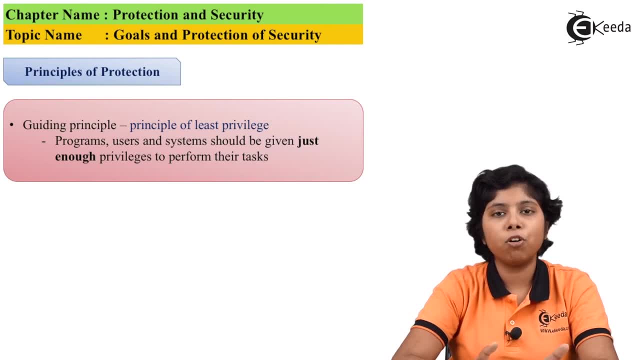 can uses a stack and buffer overflow to buffer overflow of that particular process and reach the process management area. so whenever we reach the process management area it will have a section known as a privilege. so there the list of this privileges are mentioned for the particular user. it then reaches by overflowing the information till there. 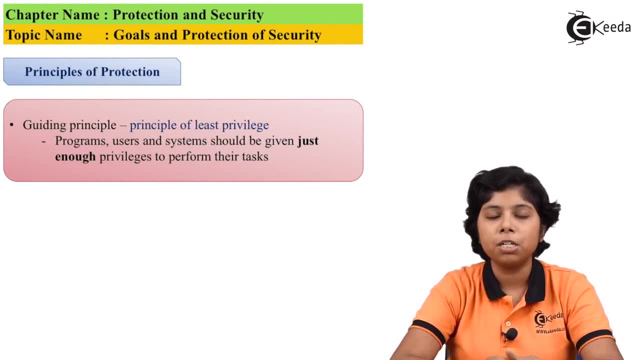 and then changes the privileges to maximum to get and file access in an intruded way. so the operating system protects this list privileges. that is, that when a user needs to access a file, a particular privilege is given to them. so enabling of the privilege is given to. 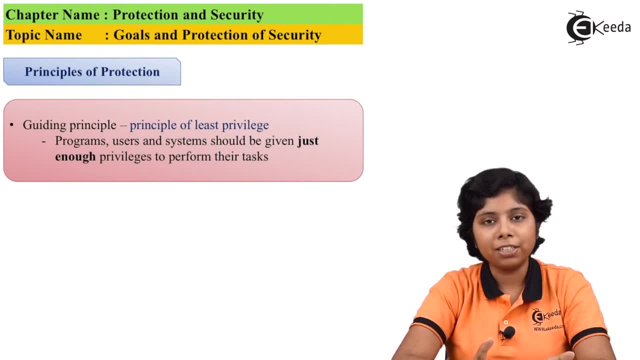 done just before the file accessing and after that the file is accessed in that particular privilege mode, again it will be disabled for the user so that no user can access habits. all privilege right by default. every user has to gain the privilege only before accessing the file. so this can be maintained by the operating system by maintaining a separate list. 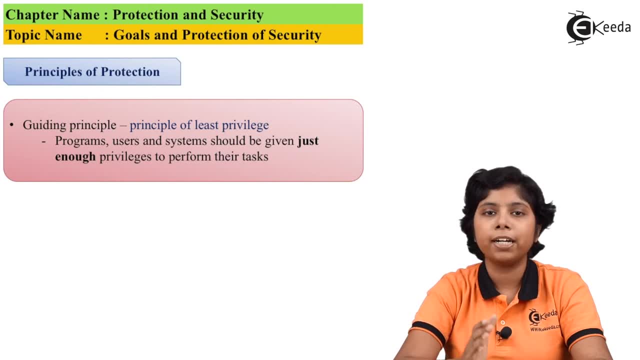 containing all the privileges that is now being attended by the user. so this separate list in this increased and decreased between this rbac- that is, a role place access control on that user, is using that particular privilege. so in this way we can maintain the principle of the list. 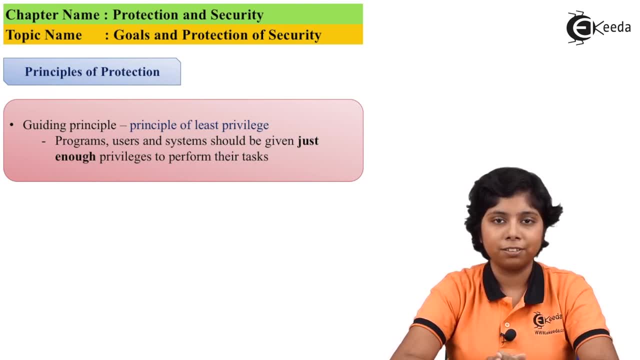 privileges for protecting an environment. now, computers implemented in a computing facility can give us this list, privileges, principles, accordance, and we can use it to create a list of privileges for protecting an environment. and we can use it to create a list of privileges for protecting an environment that, whenever this computing facility is done, only specific services on the network. 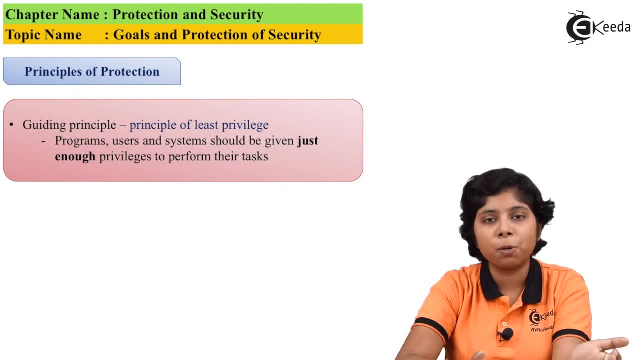 service or a remote operation that the remote patient is performing, specific system calls under the specific services only. so if the specific service is not mentioned to the rpc of that remote operation then this specific privilege is not given to the remote user. so according to again scl and the specific service system calls, it is maintained. protection of the. 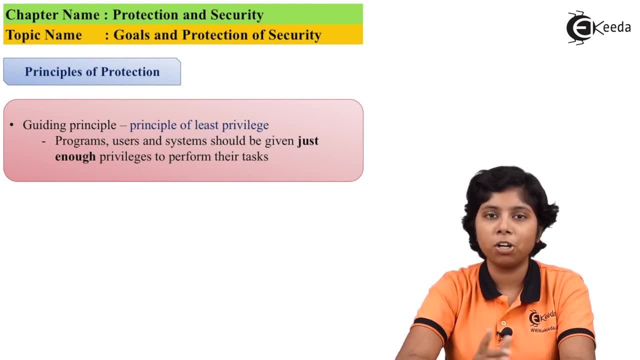 list privileges while the remote operation is being performed on a client server site. now, if we come to the operating system performance, we can say that the least principles of these privileges is mentioned between these variations of operating system. for windows, it maintained a maximum privileges as possible, given to the user, very least protection. 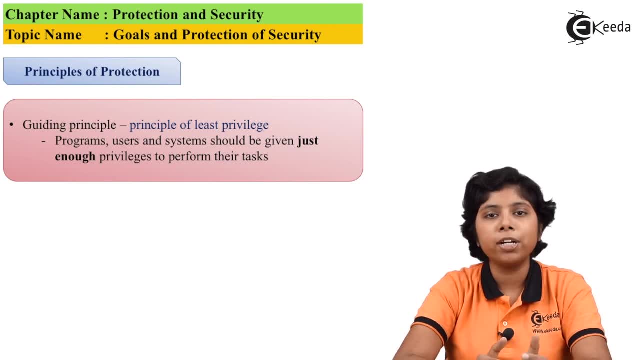 about them. comparing to it, solaris has a more intended protection than windows, but as it is a variant of the UNIX which was earlier taking a very little protection about these privileges. but nowadays Solaris uses a sequence of binary arrays which is used to protect the data at 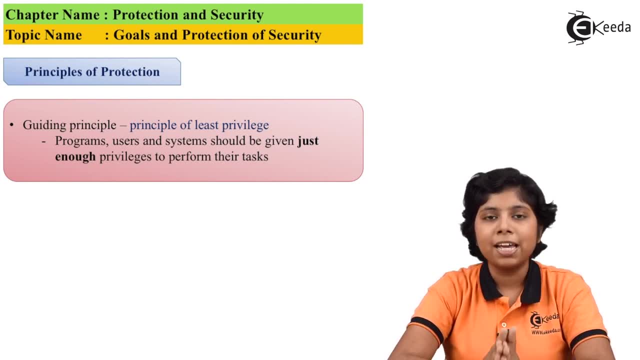 its most. So the list of principal privileges is mentioned in Solaris at the most, then Windows and then any other operating system. But Windows has more protecting environment than Solaris, but actually they are less computationally feasible than the Solaris one. So it is not.